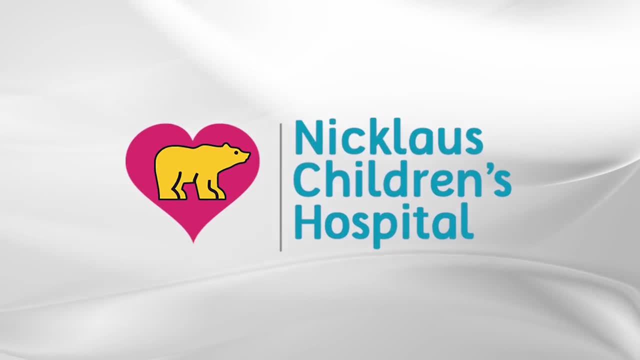 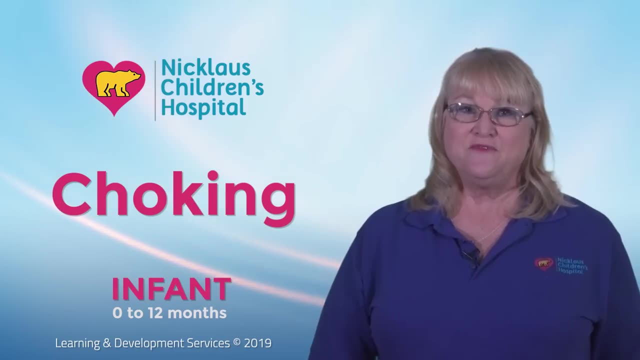 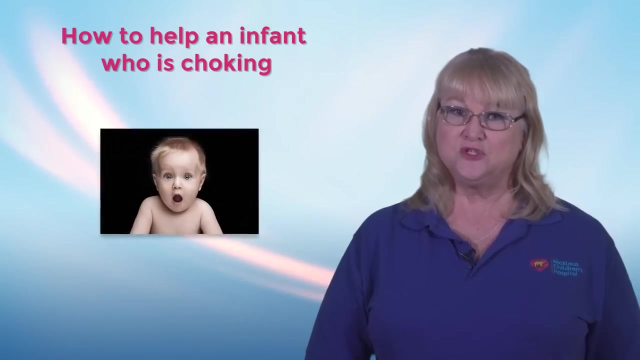 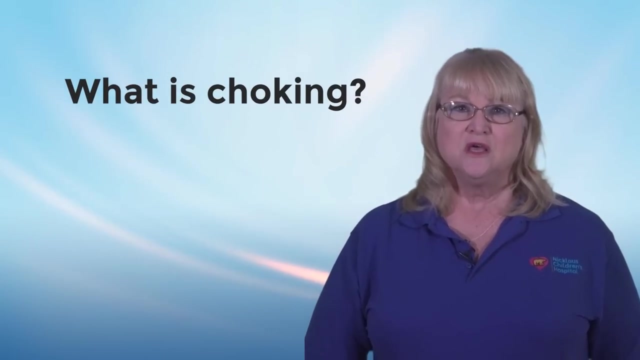 Hello and welcome to Nicholas Children's Health System Learning and Development's choking educational video. I'm Linda and I will demonstrate how to help an infant who is choking. If choking is severe, CPR may be required. What is choking? Choking means something such as food or an object has gotten stuck in the airway. preventing 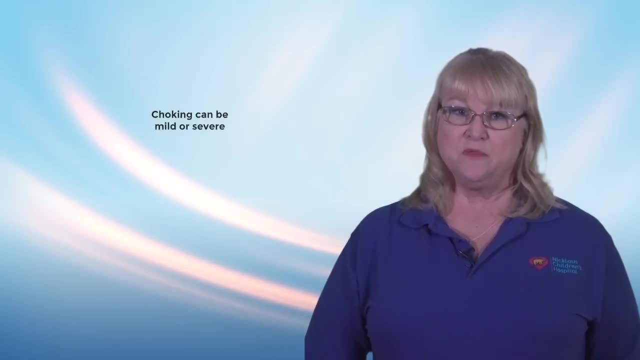 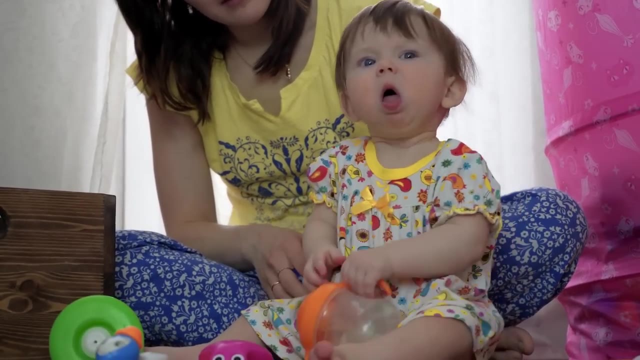 air from getting into the baby's lungs. Choking can be mild or severe. Mild choking means that the baby can cough and make sounds. If the baby is coughing, let them cough. They're trying to get the object out, But if you're worried about the infant's breathing at 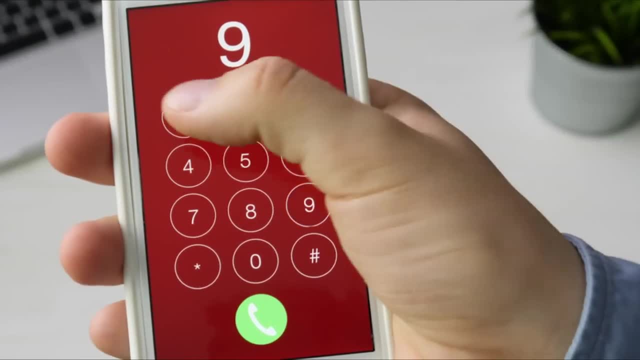 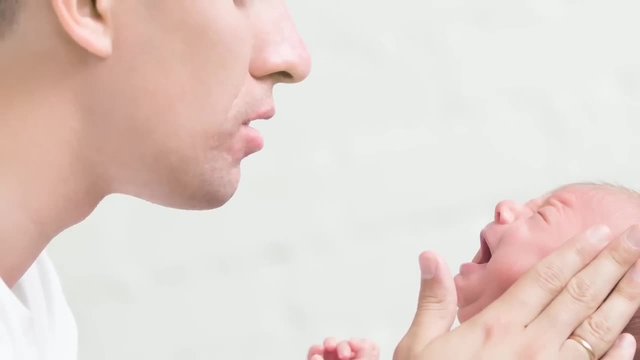 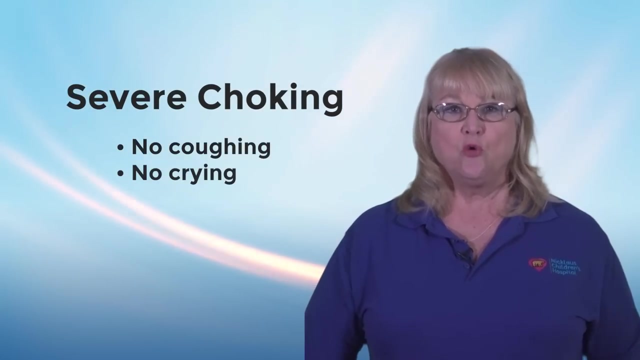 any time, do not hesitate, Call 911.. Severe choking means that the airway is completely blocked. The baby will panic and will not be able to breathe or make any sounds. In severe choking, there's no coughing, no crying, no sounds. Your quick response. 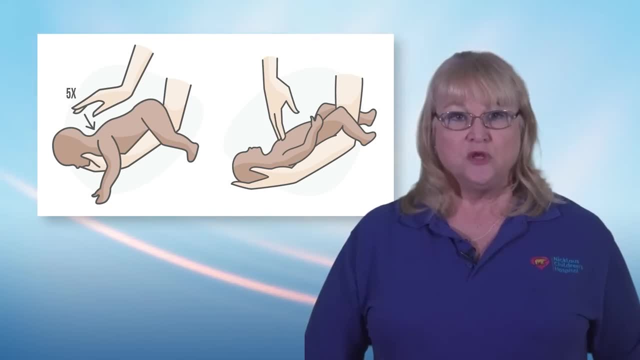 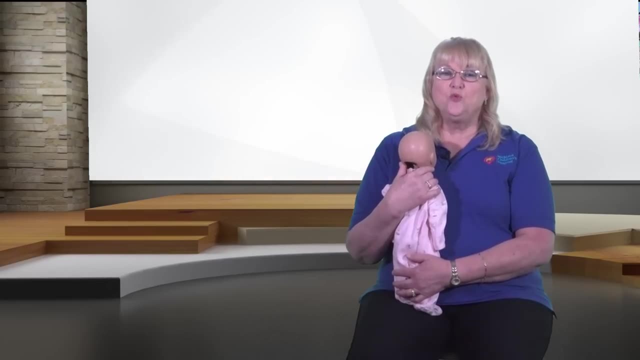 to choking can save your baby's life. You need to get the obstruction out so the baby can breathe. To get the object out, you will need to give a series of back slaps and chest thrusts. Let's start with the back slaps. 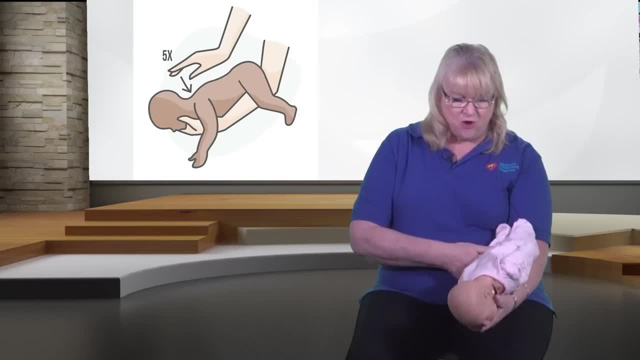 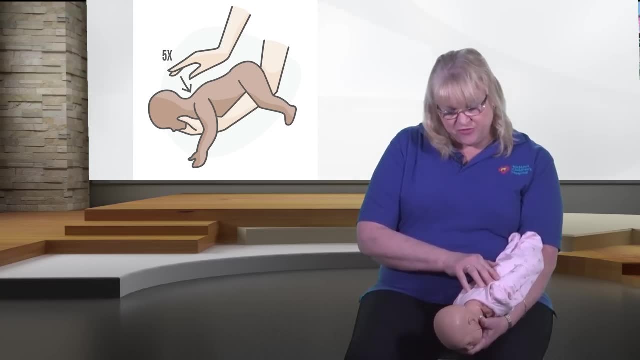 Place your baby face down over your forearm, supporting the head and neck with your hand. You may wish to sit and support your forearm on your thigh Back slaps are giving down and towards the head And we'll give a series of five. Let's try 1, 2,, 3,, 4, 5.. If the 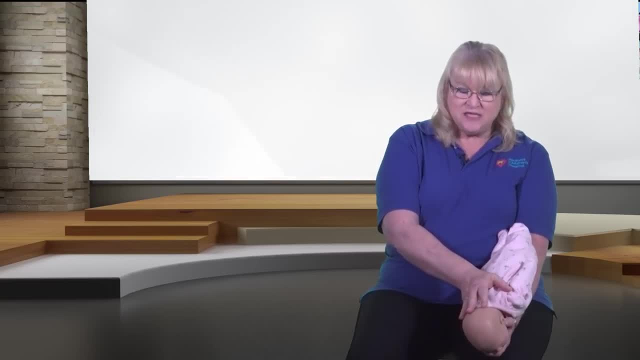 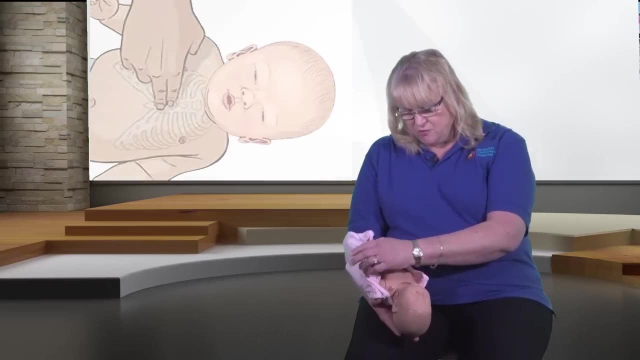 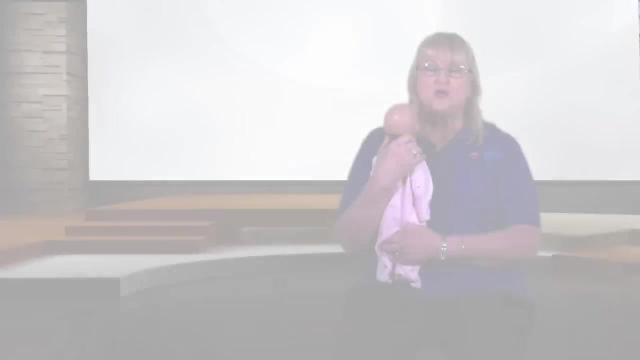 object does not come out, you'll need to pace the baby face up. Support the baby's head and neck with your forearm. Place two fingers just below mid-nipple line over the center of the chest and give five chest thrusts. Try with me. Place your baby face down over your forearm, supporting their. 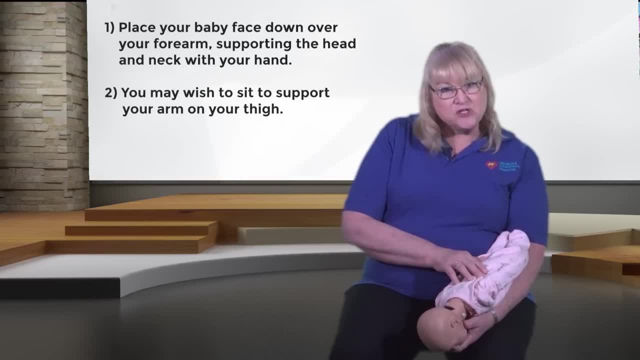 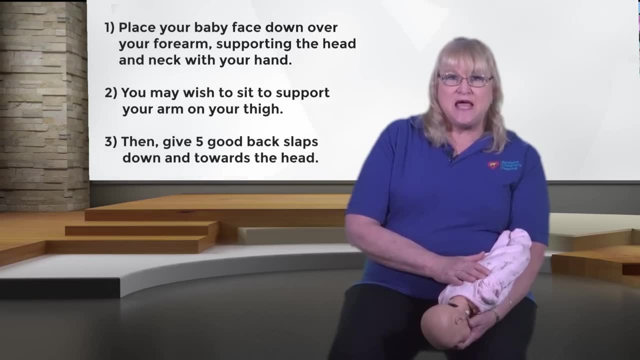 head and neck with your hand. You're going to maybe wish to sit so you can support your forearm on your thigh. Then give five good back slaps down and towards the head, right between the baby's shoulders. Nah, nah, nah, scope. 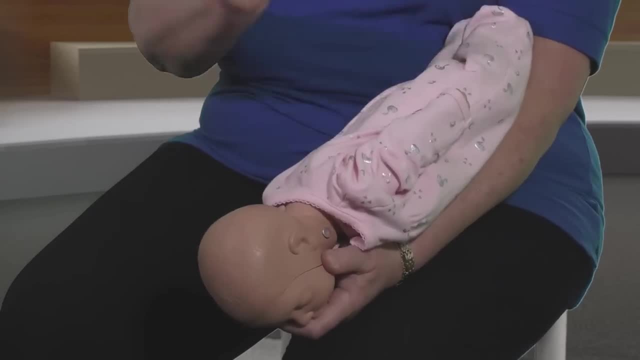 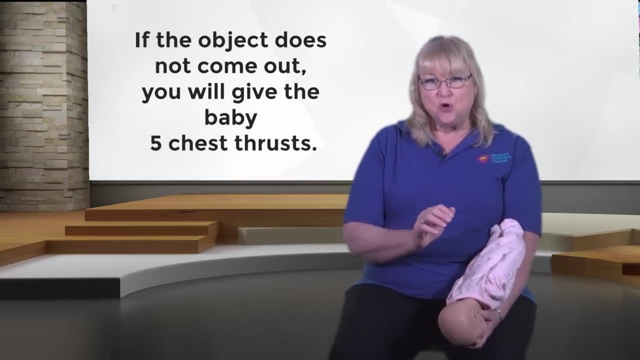 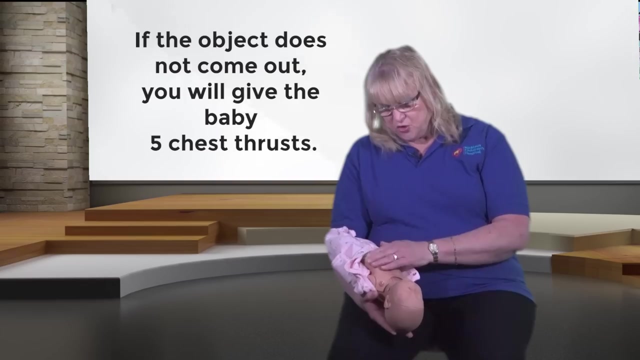 The chest is going to deliver 5 chest thrusts. Arrange your hand on the shoulder blades as you pull them forward: 1,, 2,, 3,, 4, 5.. If the object does not come out and the baby is still squirming, turn. 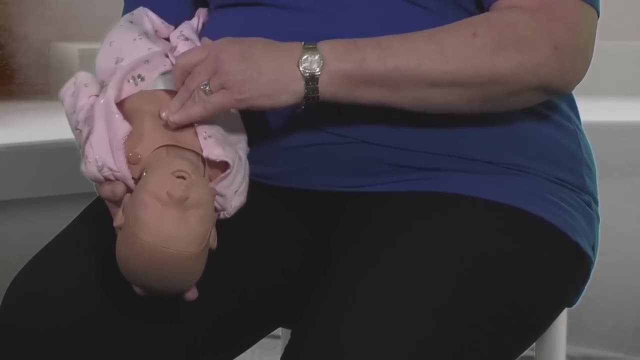 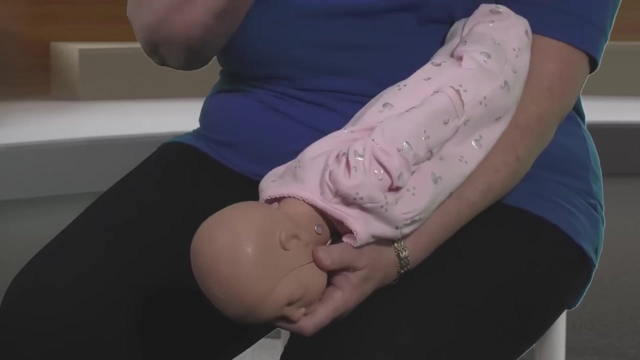 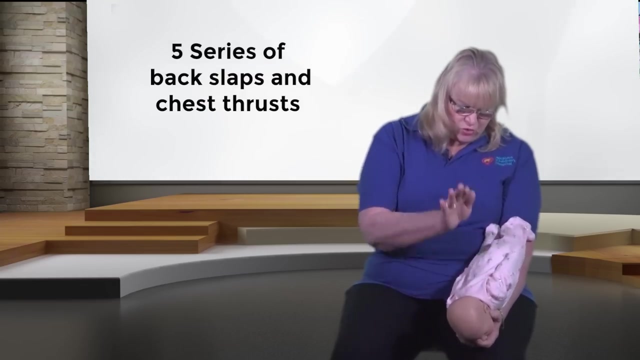 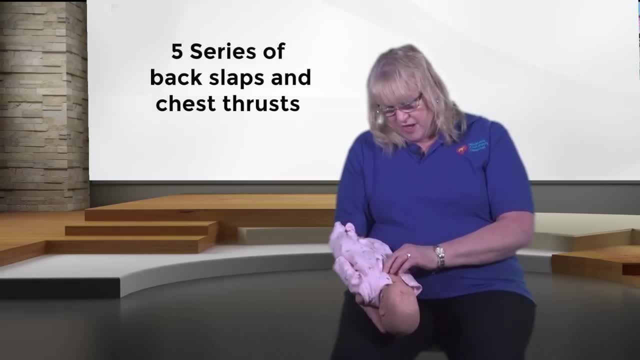 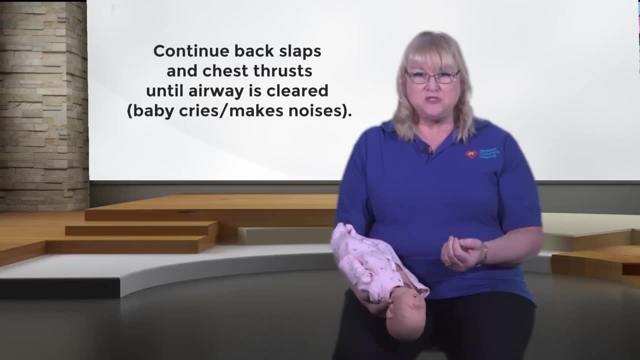 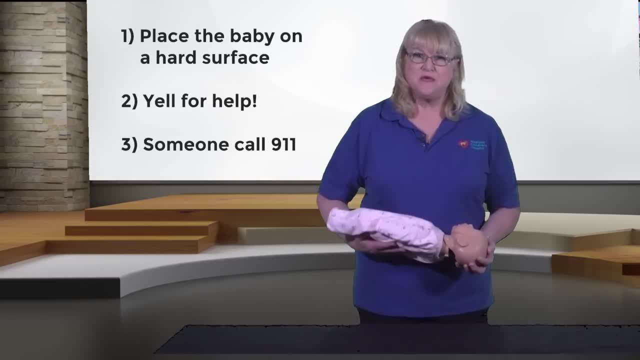 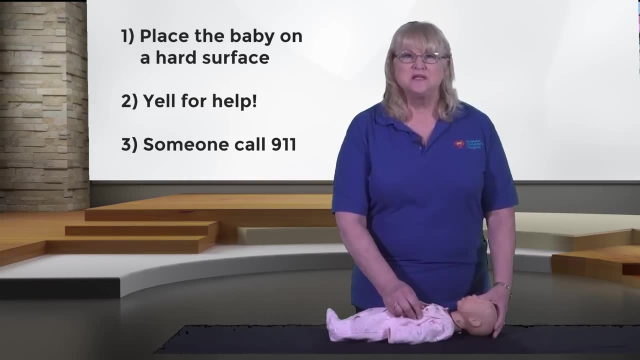 unresponsive and floppy in your arms. place the baby on his or her back on a hard surface such as the table or the ground. Yell for help, Help, Help Someone. call 9-1-1.. Hey, you in the blue shirt. call 9-1-1.. If you're alone, you'll need. 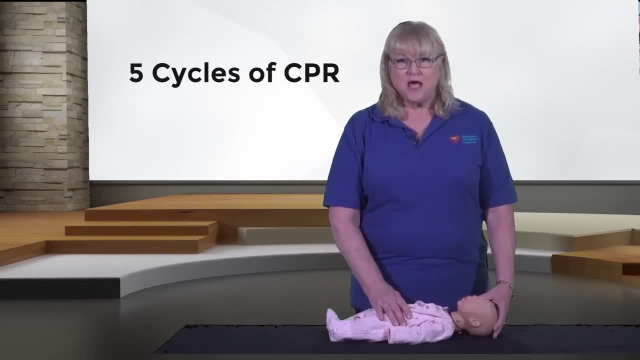 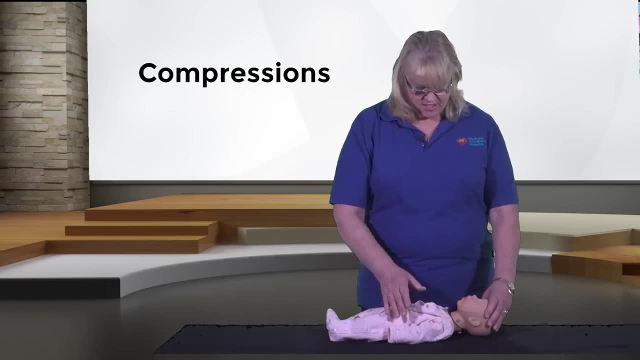 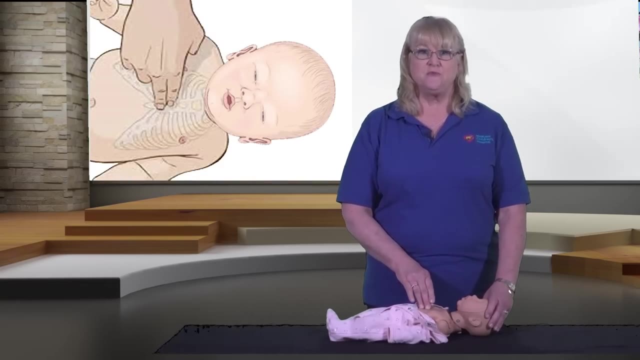 to give five cycles of CPR. Don't hang up. Put the phone on speaker so emergency staff can help you. We're going to start with compressions First. you're going to find your hand position two fingers just below mid nipple line, in the center of the baby's chest. Push hard and fast Count. 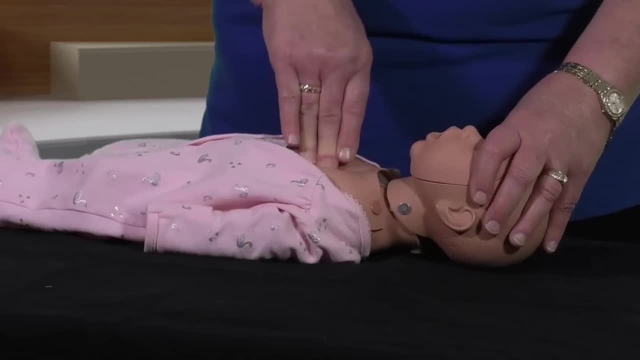 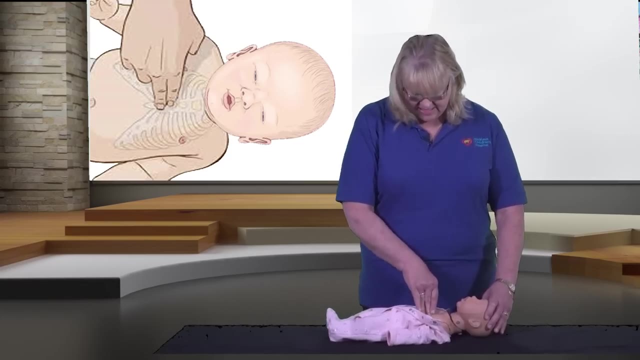 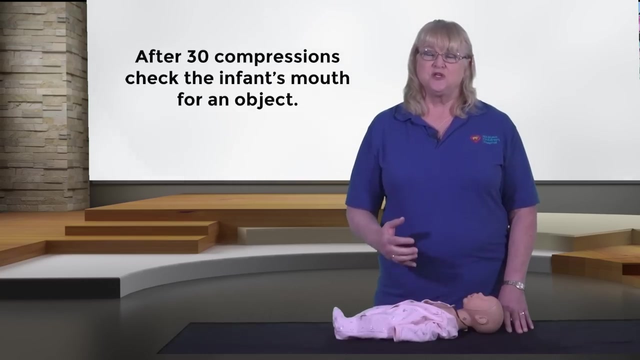 out loud to a count of 30: one, two, three, four, five, six, seven, eight, nine, ten, 11, twelve, thirteen, 14, 15, 16, 17, 18, 19, 20, 22, 23, 24, 25, 25, twenty-six, twenty-seven, twenty-eight, twenty-nine, thirty. After 30 compressions, you'll need to check. 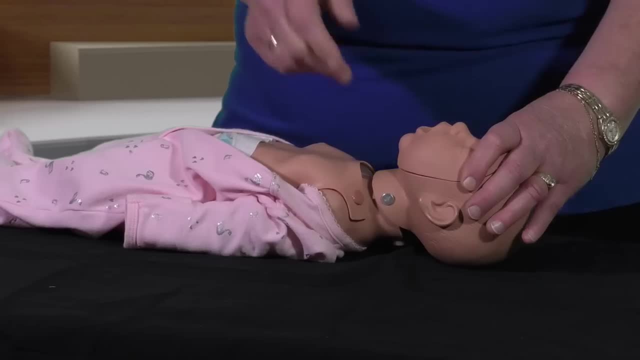 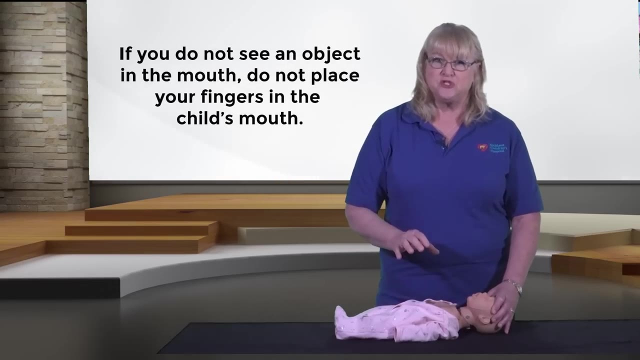 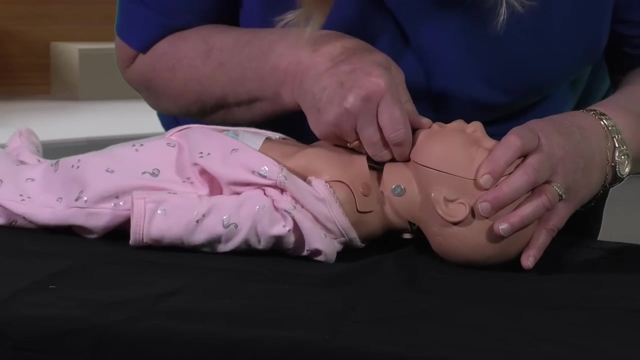 the infant's mouth to see if the object has come forward. If you see an object, take it out. If you don't see it, do not place your fingers in the child's mouth. You may push the object further down. Try it with me. You check the baby's mouth, Open the mouth, Look to see No objects are there? 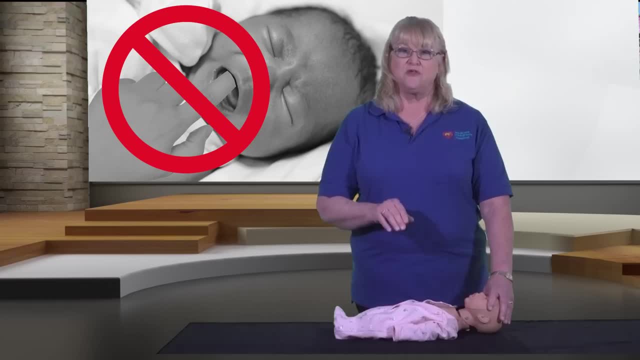 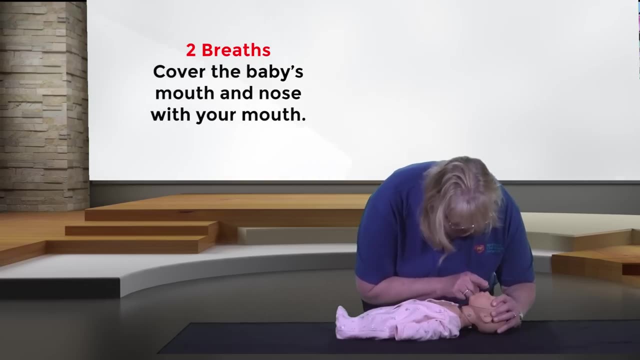 Remember, do not place your fingers in the mouth if you do not see an object, If nothing is there, you're going to attempt to give two breaths, Cover the baby's mouth and nose with your mouth and give two little puffs, hoping to see the chest rise. 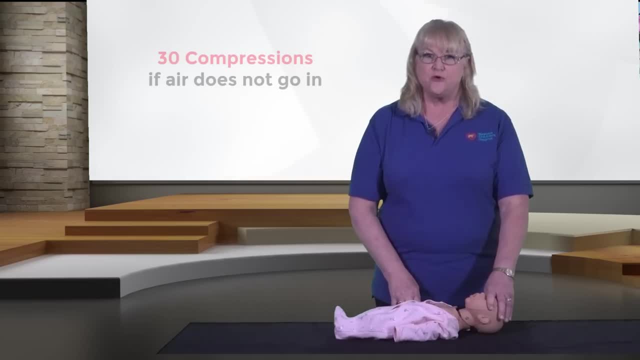 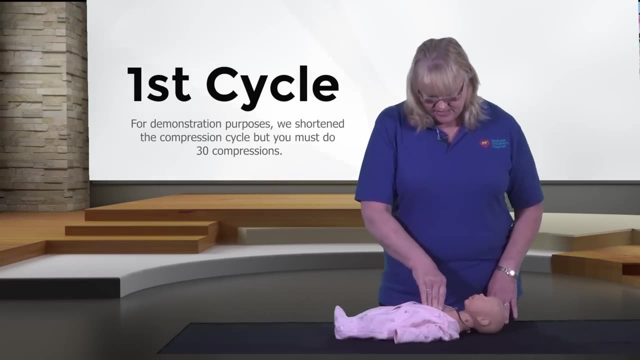 If air does not go in, we'll need to complete the 30 compressions and breaths again. Let's try it as a set: One, two, three, four, five, twenty-six, twenty-seven, twenty-eight, twenty-nine. 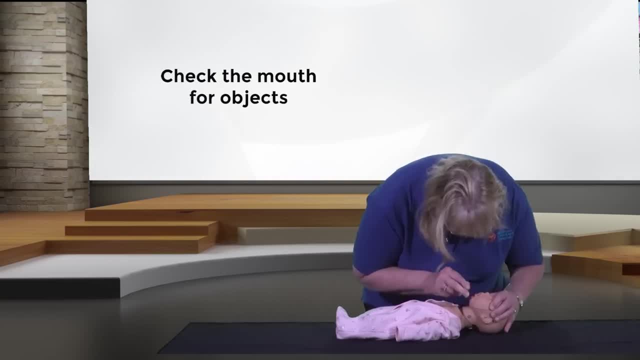 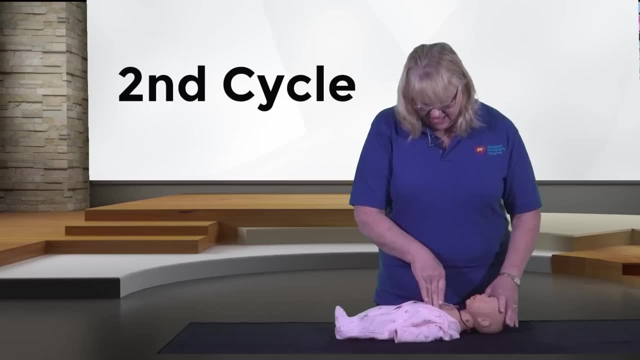 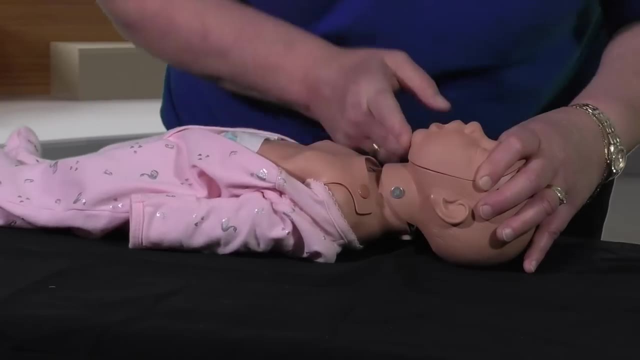 thirty. Check the mouth. Do I see anything? No, Attempt to breathe. Air does not go in. Repeat One, two, three, four, five, twenty-six, twenty-seven, twenty-eight, twenty-nine, thirty. Check the mouth. Attempt to go in. Air does not go in. Repeat One, two, three, four. 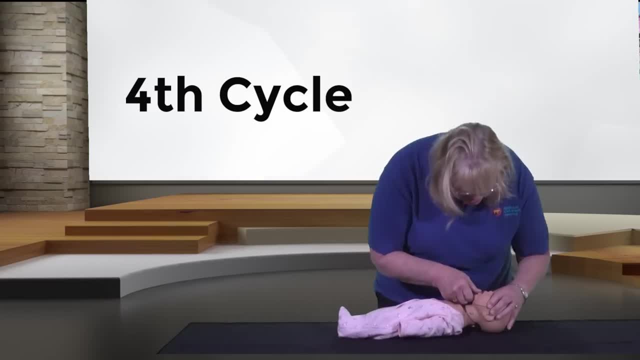 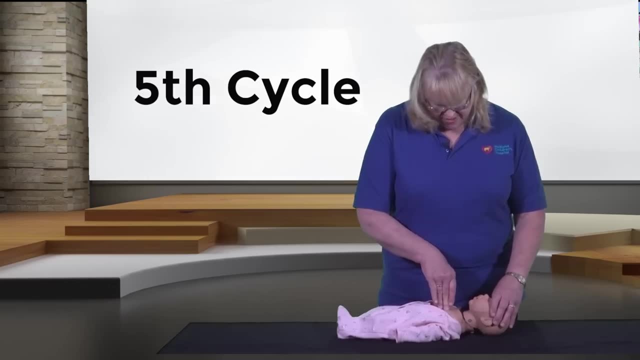 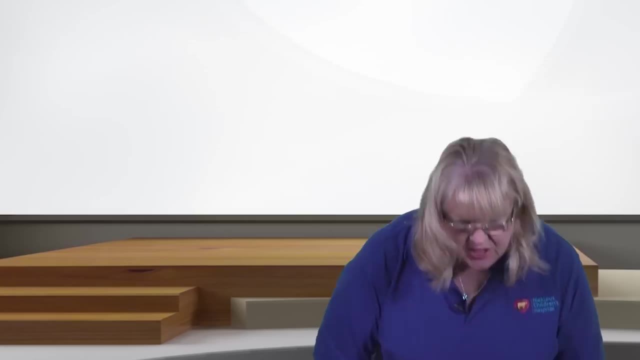 five, twenty-six, twenty-seven, twenty-eight, twenty-nine, thirty. Check the mouth. Nothing. Try to breathe. Air does not go in. Repeat One, two, three, four, five, twenty-six, twenty-seven, twenty-eight, twenty-nine, thirty. Check the mouth. Attempt to breathe. Continue giving compressions. 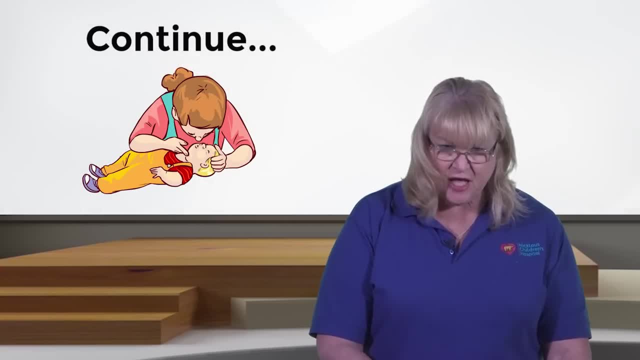 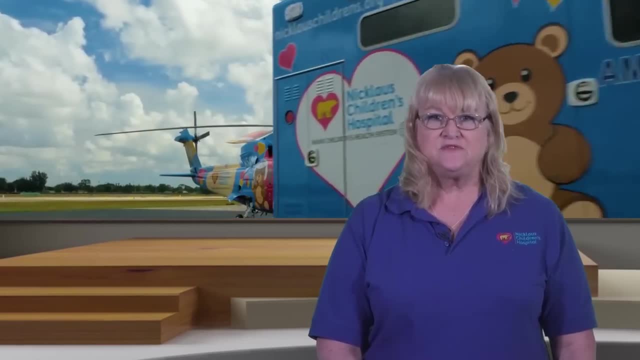 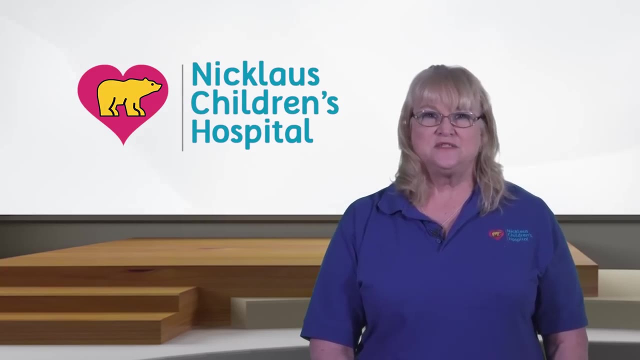 checking the mouth and attempting to breathe until the object comes out, the baby wakes up, cries or coughs, or to emergency personnel arrives to assist you. This completes How to Help an Infant Who is Choking. On behalf of all of us at Nicholas Children's Hospital, we thank you for joining us. 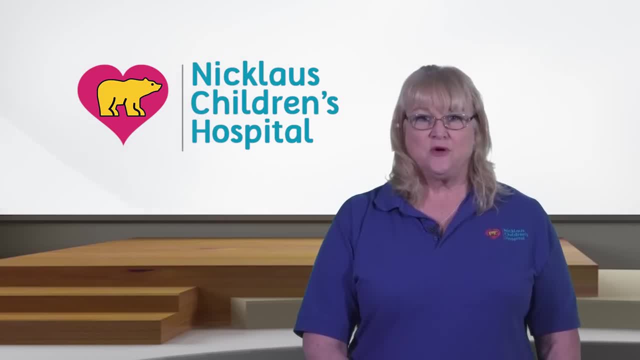 We hope you found this instructional video helpful. Thanks for learning with us.